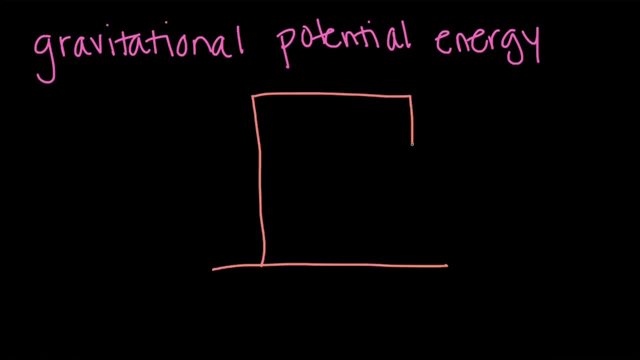 where potential energy is zero. Consider a book on a bookshelf. If the book is on this shelf, we can use this shelf as the zero point for potential energy. Moving it to a higher shelf would mean it has gravitational potential energy relative to that lower shelf. 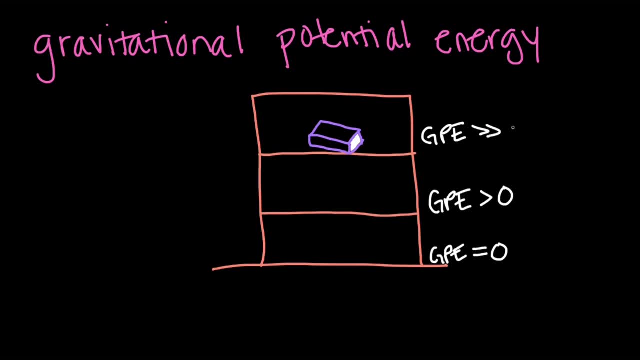 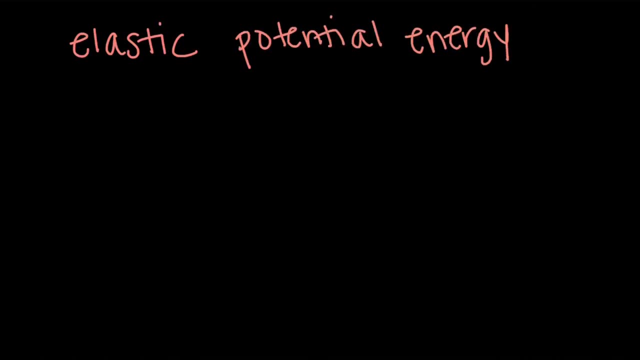 Or relative to the floor, if we want to use that as our comparison. Next, we have elastic potential energy, which is the potential energy some objects have due to their shape being changed. These types of objects are called elastic objects. Elastic objects are made. 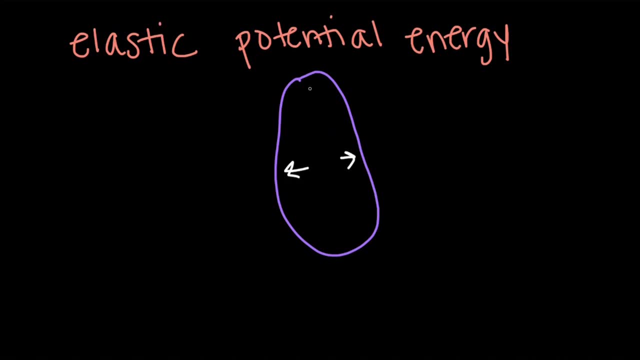 of materials and designed so they have internal or inside forces that try to return them to their original shape. One very common example of this is a spring. When you stretch or compress a spring, you change its shape, and the shape of the spring causes internal forces that try to return the 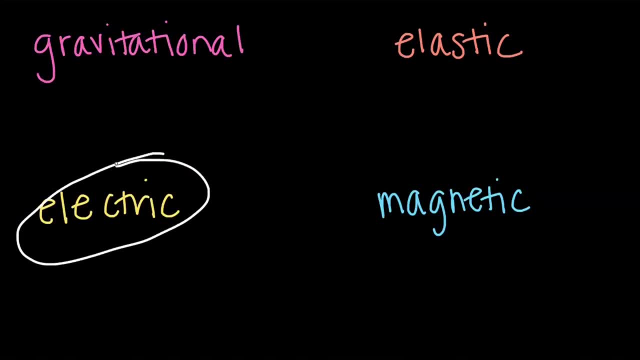 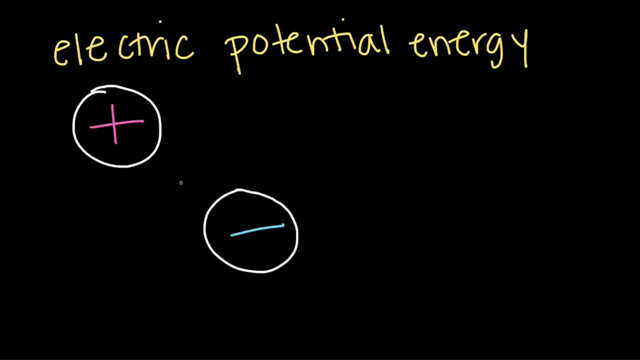 spring to its original shape Now: electric potential energy, which is the potential energy a charged object has due to the electric force from another charged object. Opposite electric charges are attracted to one another and similar electric charges are repelled. so the potential. 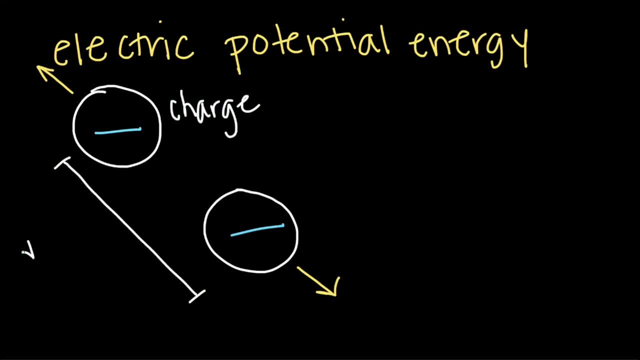 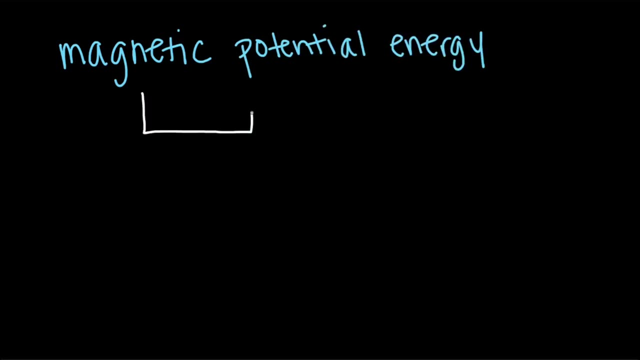 energy depends on what type of charges there are and how far apart they are. Potential energy increases when the charges move opposite the direction of the electric force, for example when two negative charges get closer together. Similarly, magnetic potential energy is the potential energy a magnetic object has due to the magnetic force from another magnet Magnetic force causes similar. 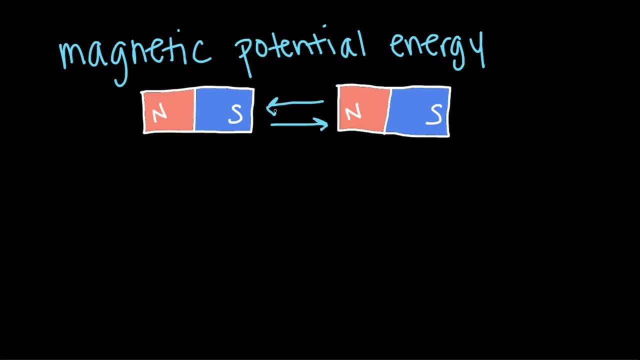 poles to repel one another and opposite poles to attract. and because magnets have north and south poles, the potential energy depends not only on the position within a field but also the magnet's orientation. Again, you could increase the potential energy by moving the magnets opposite the direction. 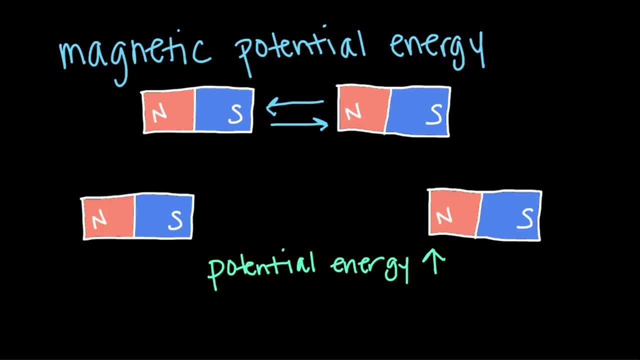 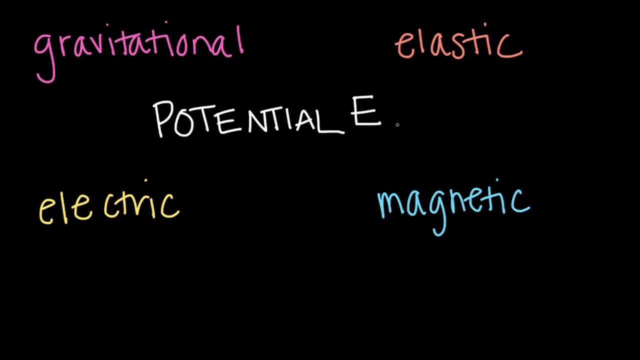 of the magnetic force, for example, by pulling apart a north pole and a south pole. All of these types of energy are due to different forces and are calculated differently, from different equations which we won't cover here. but they are all potential energy And these are.